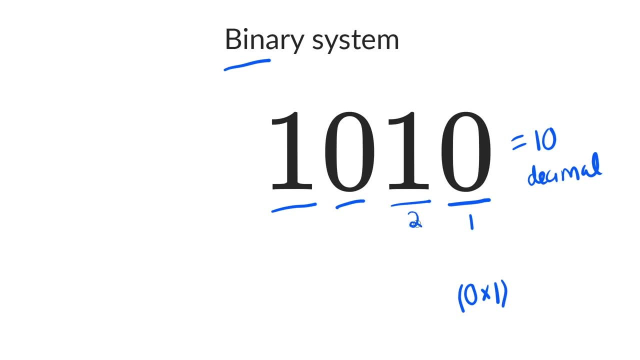 that's where things get more interesting. This is actually the 2's place, not the 10's place, And there's a 1 here, So we're going to multiply 1 times 2.. So so far this number equals 2.. The third place. 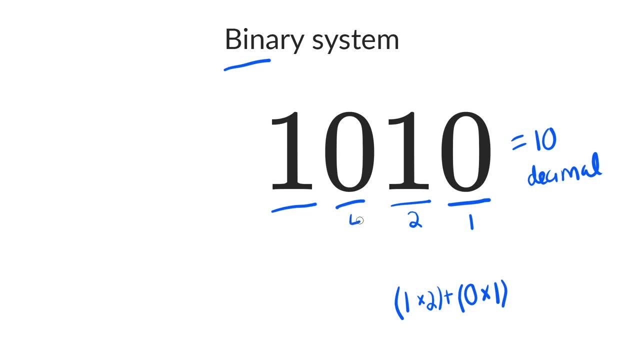 the third bit. this is 0, and this is the 4's place. So we're going to multiply 0 times 4, just once again, just 0. And we're still looking at the number 2.. Finally, this fourth. 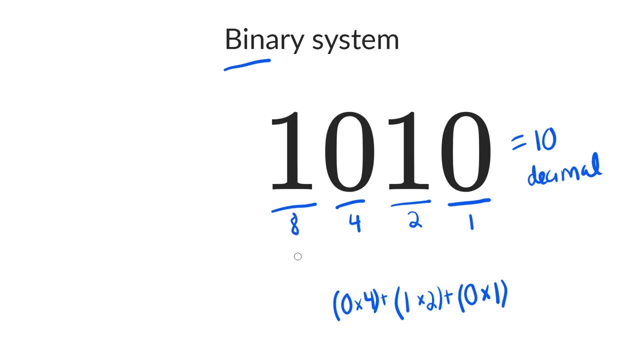 bit here. this is the 8's place and there's a 1 here, So we're going to multiply 1 times 8, add that to everything else. we end up having 8 plus 2, which equals decimal 10.. 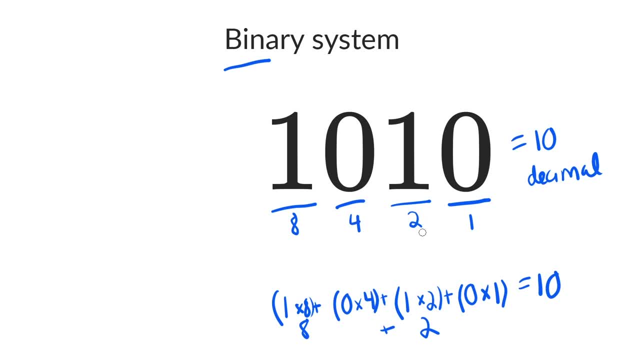 In the decimal system, each of these places represent a power of 10,, but in the binary system each place represents a power of 2.. The first bit is 2 to the 0 power. it's 1.. The second bit is 2 to the power of 1.. 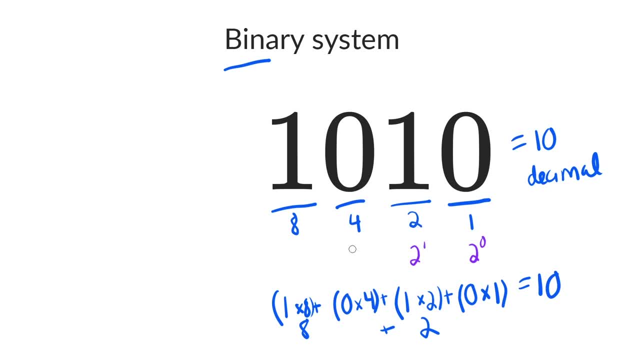 the first power, which is 2.. The third bit is 2 squared 2 to the power of 2, which is 4.. And this fourth bit is 2 cubed 2 to the power of 3.. That's 8.. That's the only difference between. 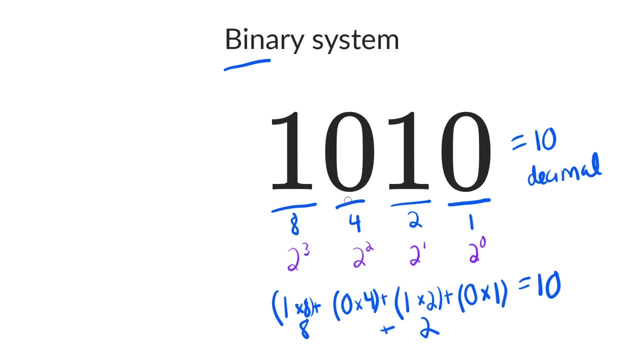 decimal and binary what each place represents. Once we know that we see what digit is in each place, we multiply them together and we get our final value. Now let's try to convert another binary number to decimal. I'm going to erase this work here, and then, for the number, let's just 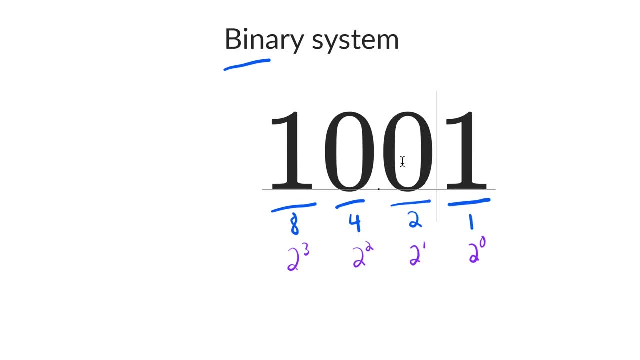 flip the bits: 0 becomes 1, 1 becomes 0, 0 becomes 1, and 1 becomes 0. What do you think this equals in decimal? I'll give you a second to think about it All. right now let's figure it out together. There's a 1 in the 1's place, So this so far. 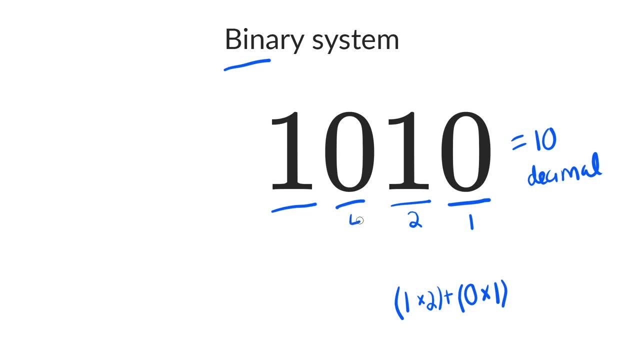 the third bit. this is 0, and this is the 4's place. So we're going to multiply 0 times 4, just once again, just 0. And we're still looking at the number 2.. Finally, this fourth. 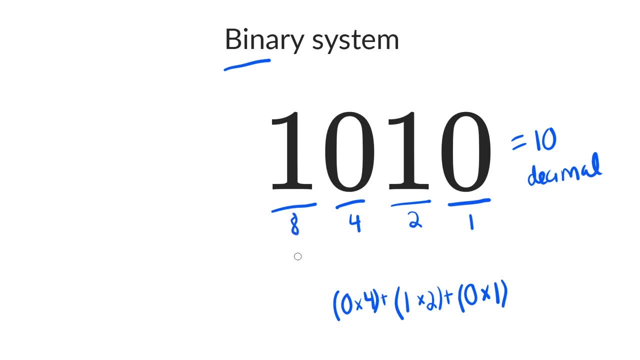 bit here. this is the 8's place and there's a 1 here, So we're going to multiply 1 times 8, add that to everything else. we end up having 8 plus 2, which equals decimal 10.. 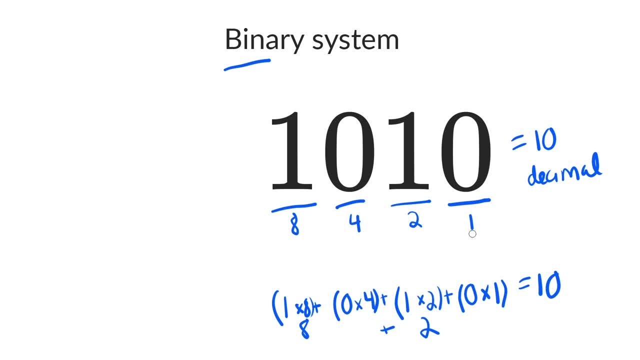 In the decimal system, each of these places represented a power of 10.. But in the binary system each place represents a power of 2.. The first bit is 2 to the 0 power. it's 1.. The second bit is 2 to the power of 1.. This is the 1's place and this is the 4's place. So we're getting this 1, and then the 3's place, and then the 4's place, and then the 2's place. So we're going to multiply 1 times 8,. add that to everything else we end up having. 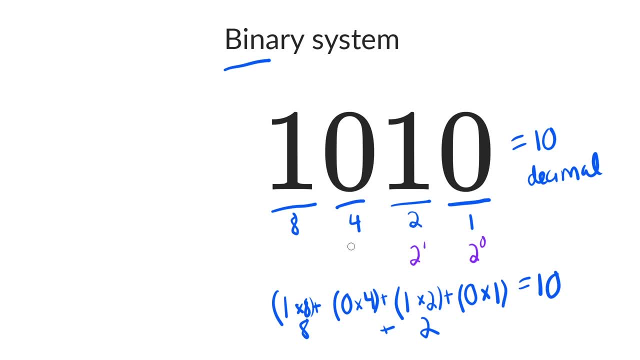 1, the first power, which is 2,. the third bit is 2 squared 2 to the power of 2, which is 4, and this fourth bit is 2 cubed 2 to the power of 3,, that's 8.. That's the only difference between. 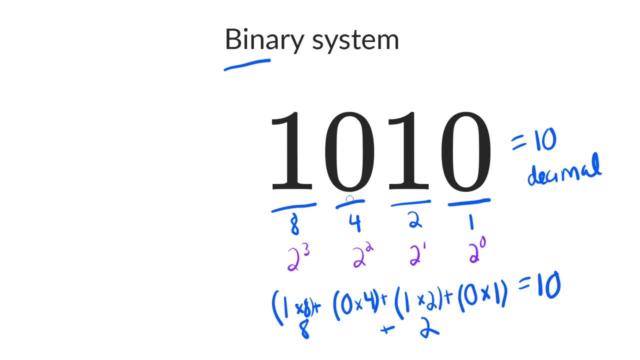 decimal and binary what each place represents. Once we know that we see what digit is in each place, we multiply them together and we get our final value. Now let's try to convert another binary number to decimal. I'm going to erase this work here, and then, for the number, let's just 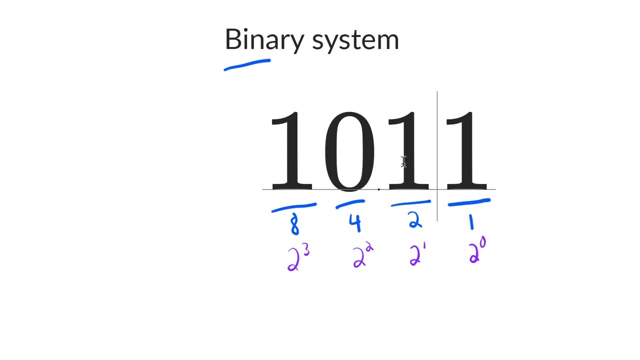 flip the bits: 0 becomes 1, 1 becomes 0, 0 becomes 1, and 1 becomes 0. What do you think this equals in decimal? I'll give you a second to think about it All. right now let's figure it out together. There's a 1 in the ones place, so this so far. 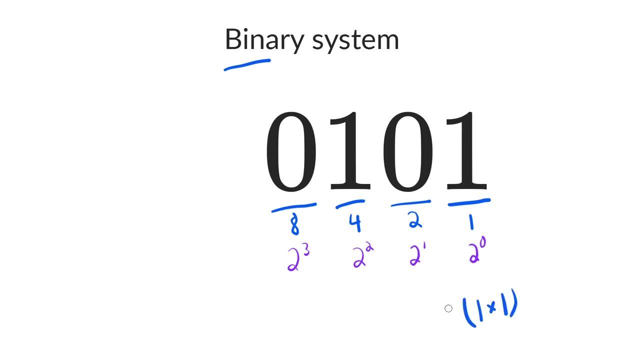 equals 1 times 1, that's 1.. There's a 0 in the twos place, so we add 0 times 2, that's 0.. There's a 1 in the fours place, so we add 1.. 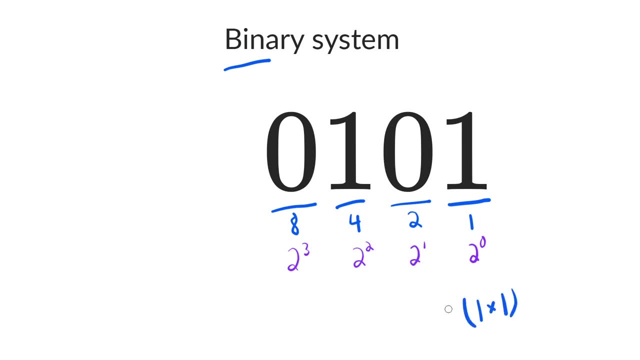 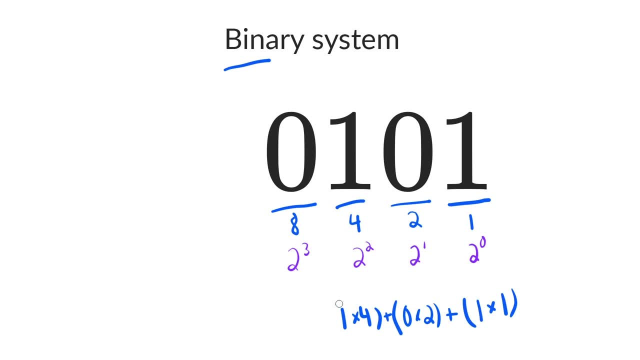 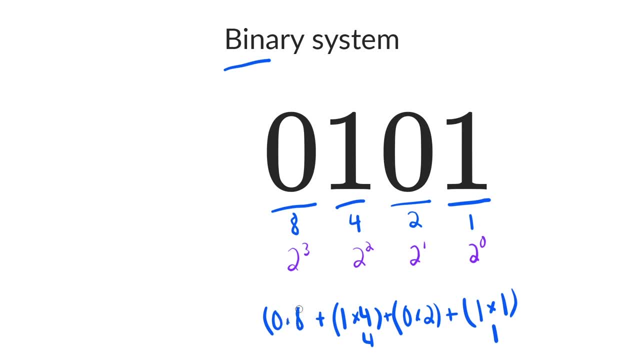 the final place, the 8's place. So that's 0 times 8, or 0.. So we've got 0 plus 4 plus 0 plus 1, which equals 5 in decimal. Let's try converting a bigger binary number to decimal. 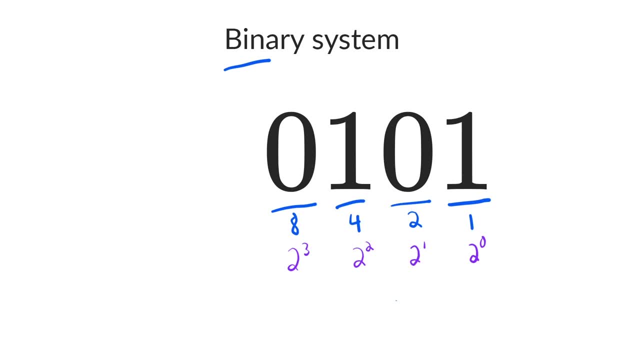 We know that this equals 5.. What happens if we add four more digits to the left of these four digits? Let's start by figuring out what each place represents. One way of doing that is just to double the previous places. So this place here is 16.. This place is 32.. This place is 64.. 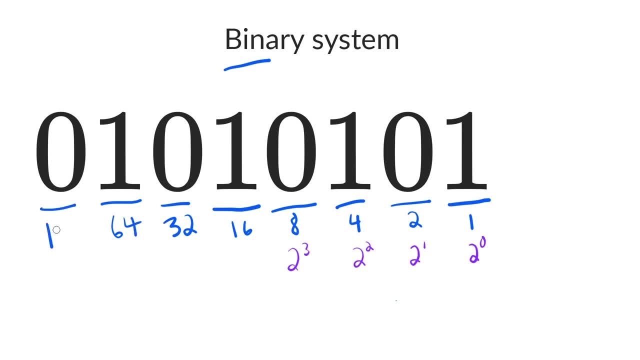 And this place is 128.. Another way of doing this is to calculate the powers of 2.. So this place is 2 to the 4th, which is 16.. This is 2 to the 5th, which is 32.. This is 2 to the 6th: 64.. And this is 2 to the. 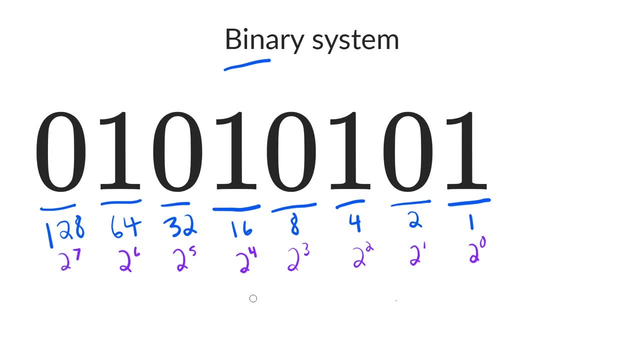 7th, 128.. Okay, so now we know what each place represents. Now we can add these numbers up. We know already that these ones equal 5.. We already did that. Now let's add in what we've added here, So we have a 1 in the 16. So that means we're going to. 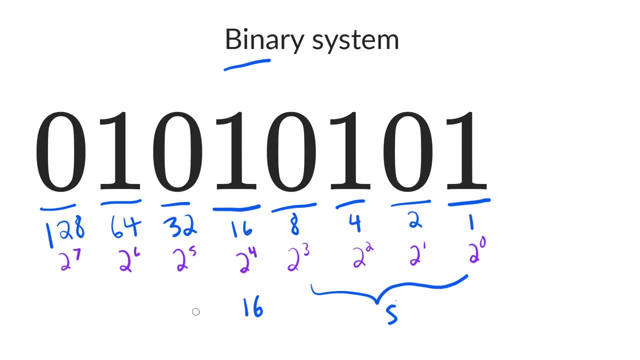 add 16 to the number, Then there's a 0 in the 32. So that's just going to be 0.. There's a 1 in the 64. So that's going to be 64. And there's a 0 in the 128. So that'll be 0. So now we've got 64 plus. 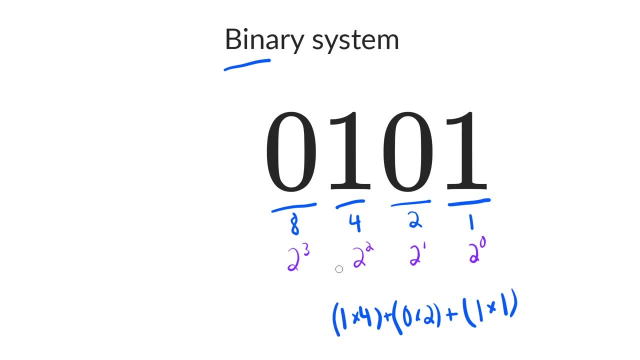 times 4, that's 4. so so far we've got 4 plus 1. and then there's a 0 in the final place, the 8th place, that's 0 times 8 or 0. so we've got 0 plus 4 plus 0 plus 1, which equals 5 in decimal. let's try. 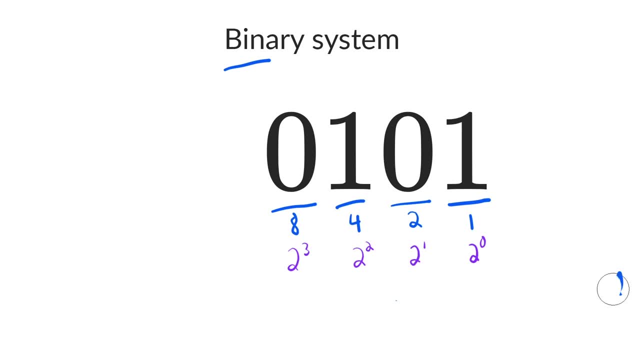 converting a bigger binary number to decimal, we know that this equals 5. what happens if we add 4 more digits to the left of these four digits? let's start by figuring out what each place represents. one way of doing that is just to double the previous places. so this place here is 16. this 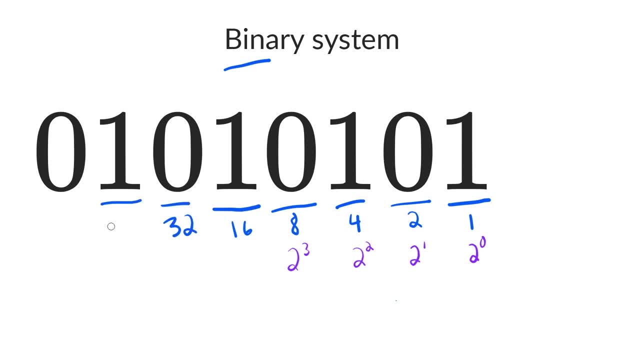 place is 32, this place is 64, and this place is 16 is 128.. Another way of doing this is to calculate the powers of 2.. So this place is 2 to the 4th, which is 16.. This is 2 to the 5th, which is 32.. This is 2 to the 6th: 64. And this is 2 to the. 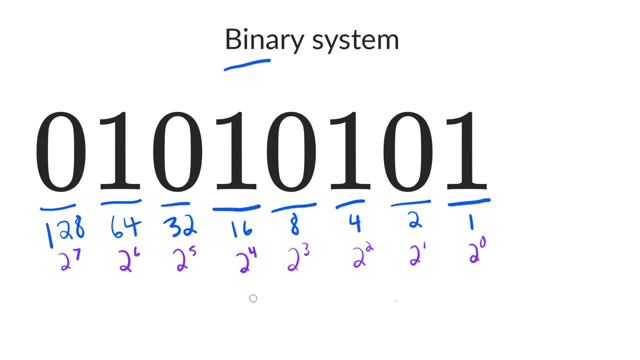 7th, 128.. Okay, so now we know what each place represents. Now we can add these numbers up. We know already that these ones equal 5.. We already did that. Now let's add in what we've added here. 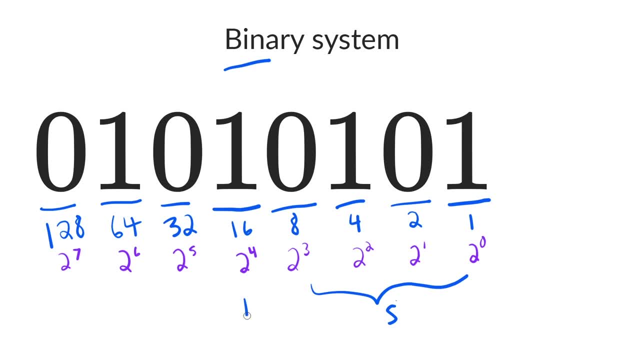 So we have a 1 in the 16.. So that means we're going to add 16 to the number. Then there's a 0 in the 32, so that's just going to be 0.. There's a 1 in the 64,, so that's going to be 64. And 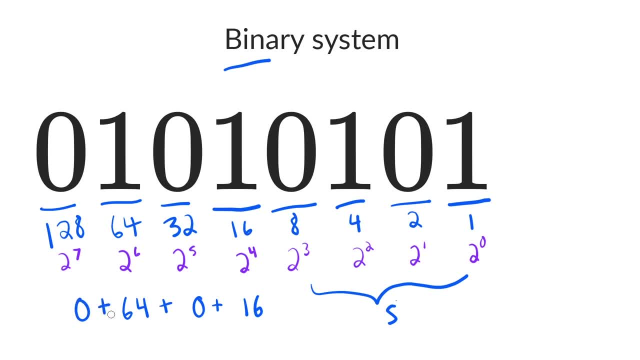 there's a 0 in the 128, so that'll be 0.. So now we've got 64 plus 64.. 16 plus 5.. So that's 80 plus 5, which is 85 in decimal. So it took us 8 bits to represent a number that only takes 2 digits to represent in the decimal.